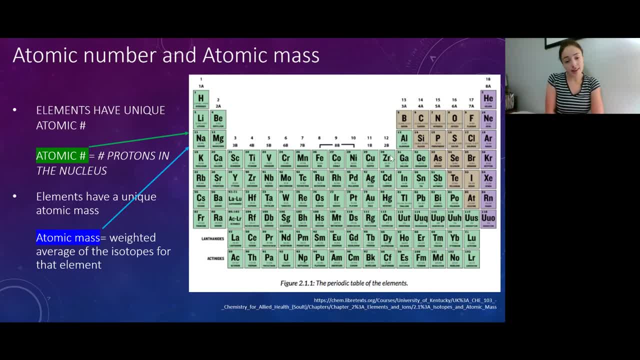 understand a little bit about atomic nuclei and isotopes. Each element has a unique atomic number. This atomic number is the number of protons and protons, And this atomic number is the number of protons in the nucleus. The number of protons is what defines an element. If you change the number, 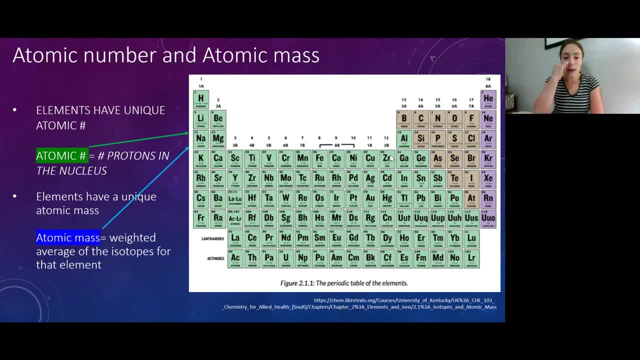 of protons. it is no longer that element. it's now a different element. However, if you change the number of electrons or neutrons, it's the same element but a different: ion or isotope respectively. The change in electrons causes ions, but we're not going to be talking about those today. We're 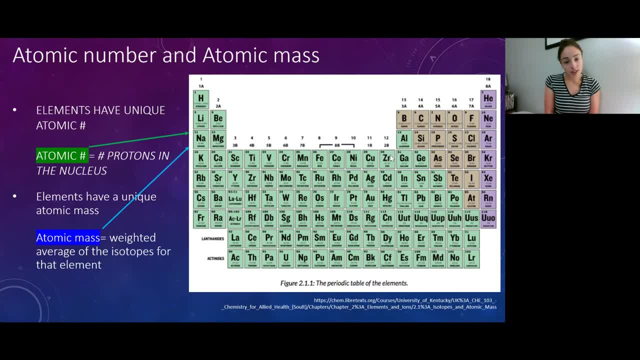 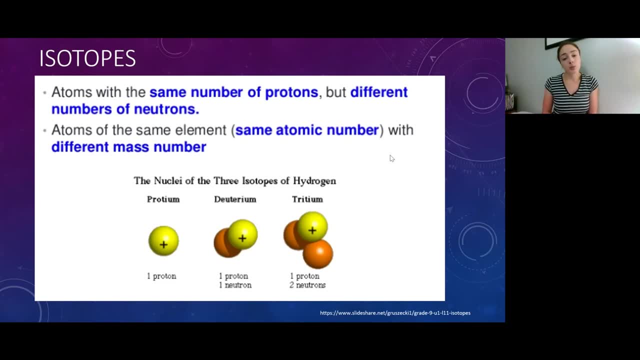 talking about isotopes, There's not always the same number of neutrons as there is protons. This is what causes isotopes to happen. Here's an example of hydrogen, which typically has one proton and one electron, And this is just showing the nucleus. The electrons are not shown in this. 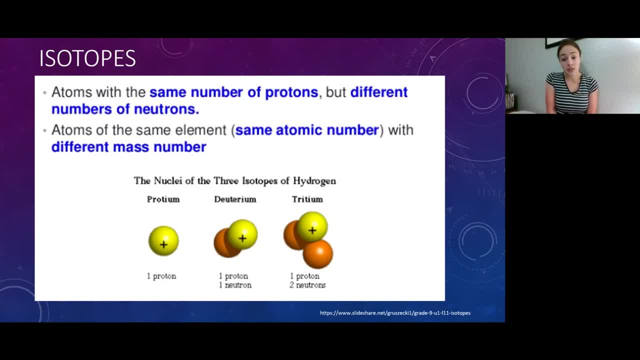 image. But if you add a neutron, it is now deuterium. If you add two neutrons, it's now triterium, And so deuterium and triterium are isotopes of hydrogen, But in this video we're 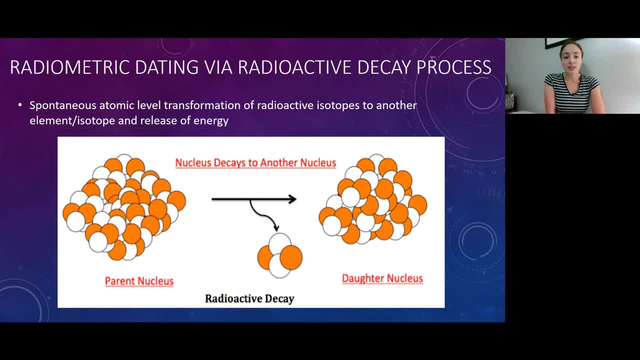 not going to be talking about all isotopes. We're only going to be talking about those that decay, And that's because this dating method is based on radioactive decay processes. This radioactive decay occurs when an isotope is unstable And wants to become stable, meaning its nucleus is unhappy with so many neutrons and protons And 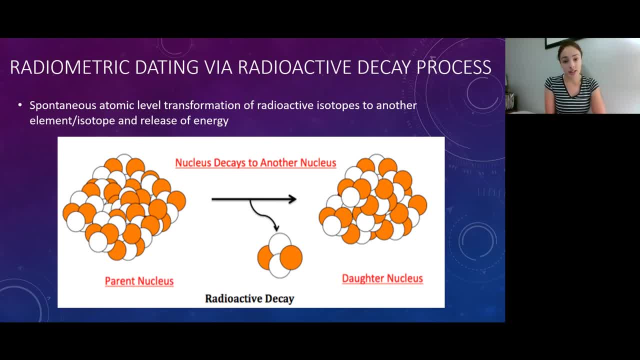 it wants to get rid of some or change some or add some, And so it's decaying into different isotopes, And the original nucleus before decay is called the parent nucleus or the parent isotope, And the product of this decay process is called the daughter nucleus or daughter isotope. 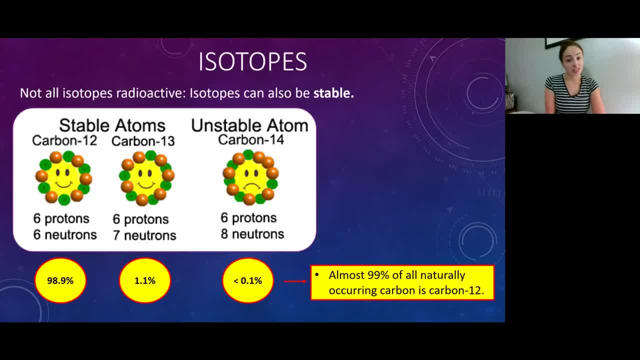 But not all isotopes are radioactive or unstable. There are isotopes that are stable, and so I thought I'd introduce this with carbon, because we will be talking about the radioactive decay of carbon-14.. However, carbon's other two isotopes, 12 and 13,, are stable, and they do not. 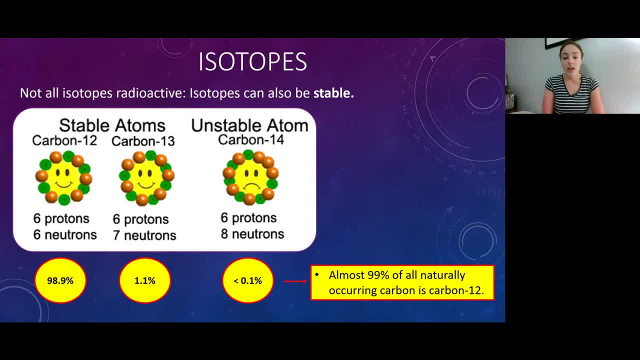 decay And so we can't use them for dating, but they are important And because of this we're going to be talking about stable isotopes in a whole separate episode or episodes, because the stable isotopes of carbon, as well as stable isotopes for other light atoms like oxygen, 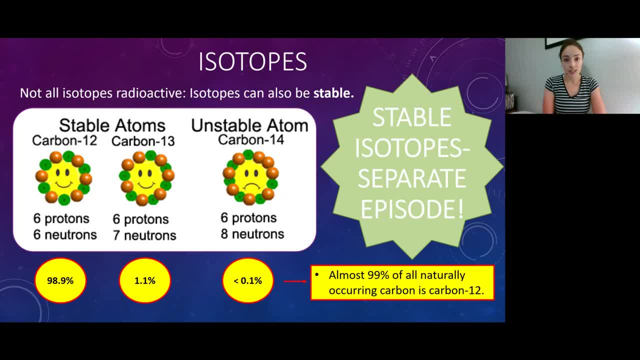 are really important for geologic reconstruction And that's why these deserve their own separate episodes. So remember that stable isotopes do exist. Not all isotopes are radioactive, However. for carbon, there is a radioactive isotope and that is carbon-14, which we will get to in later slides, But it does decay. 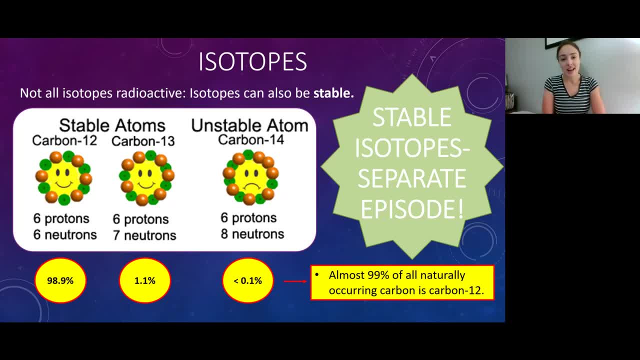 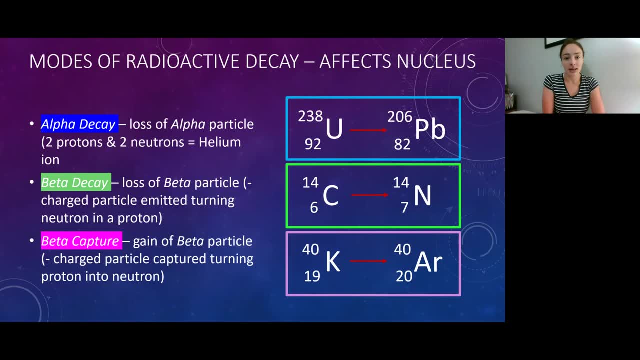 and it decays into something that's totally not carbon at all. So we'll get into how that happens. I'm going to be talking about three main processes of radioactive decay: alpha decay, beta decay and beta capture. Alpha decay can be shown by the example of 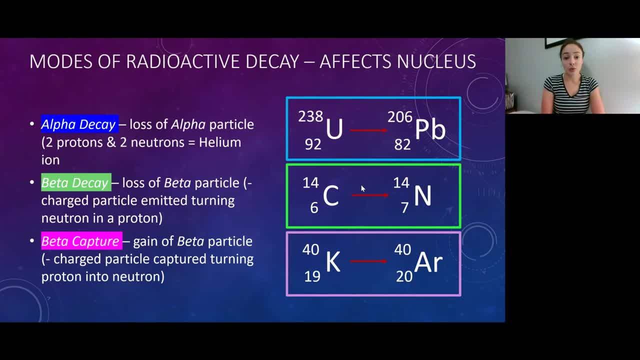 uranium-238, which decays into lead-206.. Alpha decay happens by loss of an alpha particle which is just two protons and two neutrons, or as we like to call it, helium, just because anything with two protons by definition is helium. But basically you can see here in the equations: 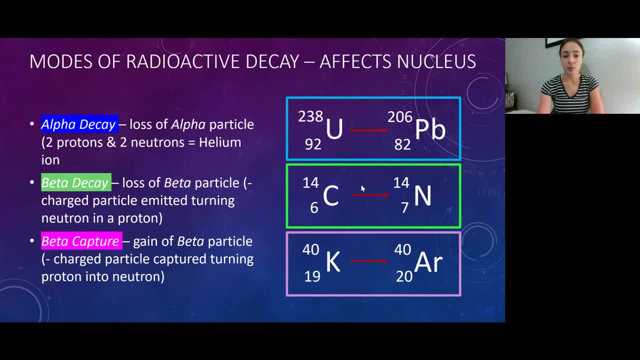 that that doesn't necessarily add up, Because if you've ever seen isotope notation, you know that this top number is the number of protons plus neutrons and the bottom number is number of protons only, And so if you're looking at this, you're going to see that the number of protons 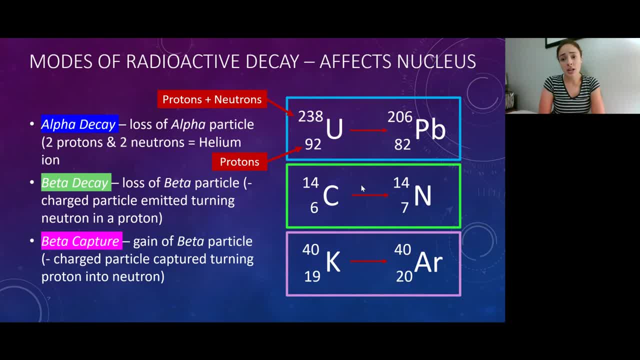 is the number of neutrons. So if you're losing two protons and two neutrons, how is it going all the way down to 82 and 206?? What the heck? Okay guys, I get it. This one's a weird one. The rest: 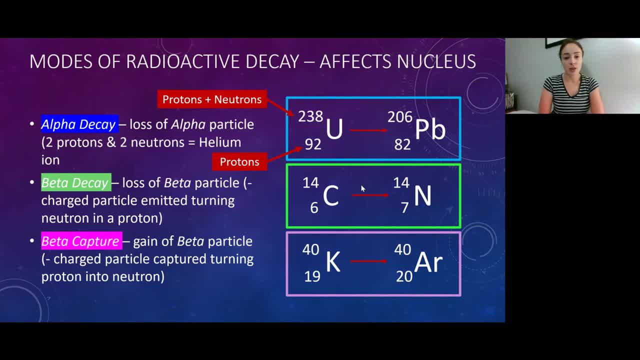 are going to be easier. The reason that these numbers go down so much for uranium decay is because uranium-238 decays over a long process. The first product of uranium decay is thorium, and then there's, I want to say, like 16 other products before you actually get to the stable. 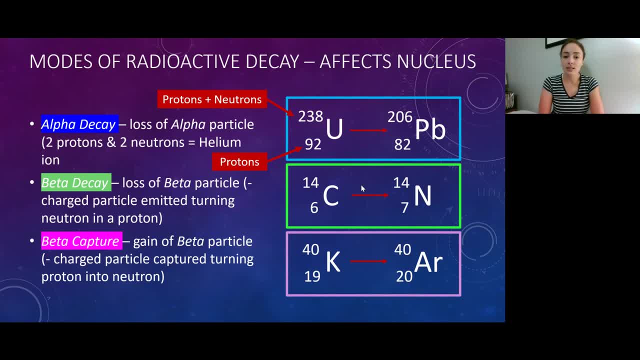 product, which is lead. The reason that these things happen in long chains like this is because sometimes, when decay occurs, the dots are not the same. So if you're losing two protons and two neutrons, that product is also radioactive, So it will decay as well, And decay will happen again. and 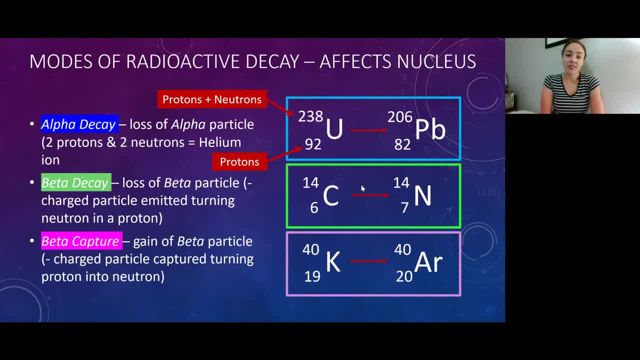 again and again, and again, until you get to a final stable product. And this is what lead is for this decay chain of uranium-238.. The next thing we'll be talking about is beta decay. Beta decay is the loss of a beta particle, which is just a negatively charged particle emitted from a neutron turning. 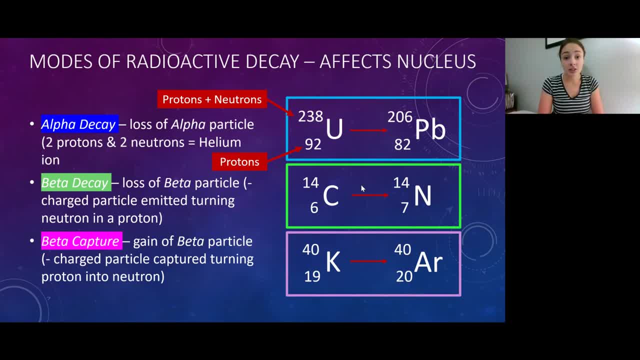 it into a proton. Yeah, I didn't know that they could do that either until I started learning about absolute dating. So if you're out there and you're wondering, holy crap, neutrons can just do that, Well, yeah, they can. So this happens in decay processes such as carbon-14. 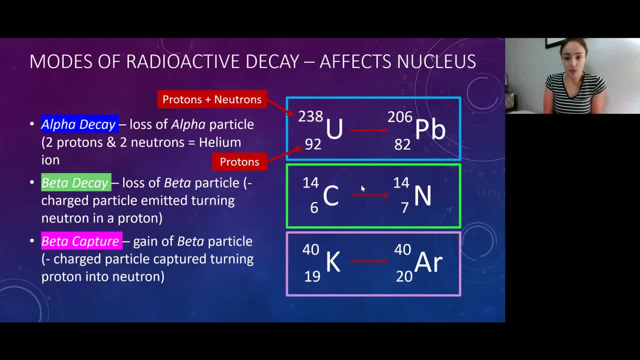 decay, Carbon-14,, which we saw was the radioactive isotope of carbon, decays into nitrogen-14.. As you can see, the proton and neutron number didn't change, which makes sense because you're not losing or gaining any protons or neutrons. It's just that one neutron is turning into a proton. 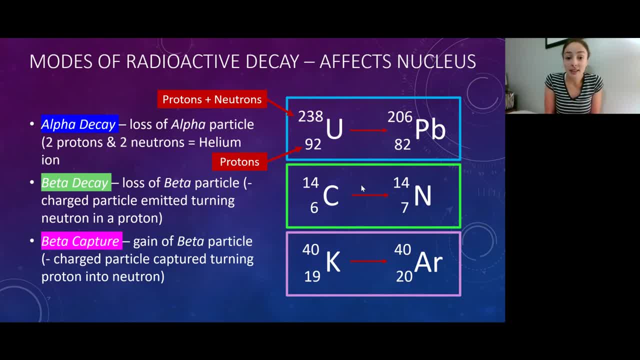 So the proton number goes up, changing the element of the isotope, which is now nitrogen, but not changing the neutron proton number. The last decay process we're going to discuss is beta capture. So this is basically the opposite of beta decay, Instead of giving away a negatively 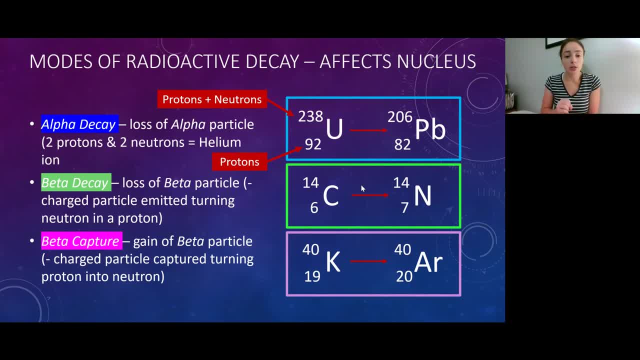 charged particle. the nucleus is actually going to capture a negatively charged particle, turning a proton into a neutron, Because the proton is positively charged. if it gets some negative charge, it'll become neutral In terms of potassium-40,. it decays into argon-40, which, as 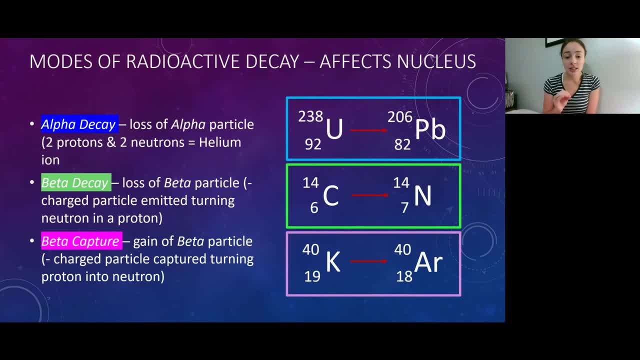 you can see, has a lower number of protons but the same number of protons and neutrons. So it's just the opposite of what we saw happen in the beta decay. Basically, the proton number went down, but a proton turned into a neutron, so a new neutron number went up and therefore the protons. 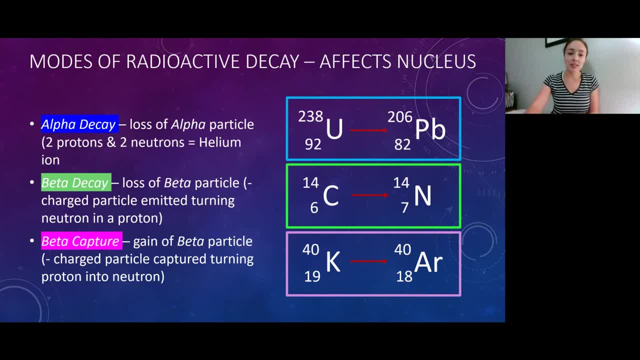 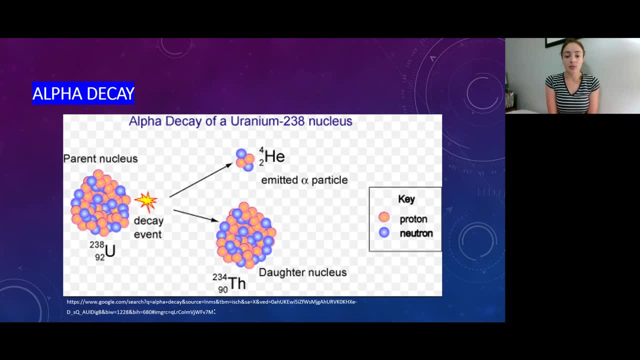 plus neutrons stay the same. Just to recap these three processes, we're going to discuss them with some depiction. In this slide you can see that alpha decay is depicted by this figure showing uranium-238 decaying into, like I said, the first product of its decay process is thorium. 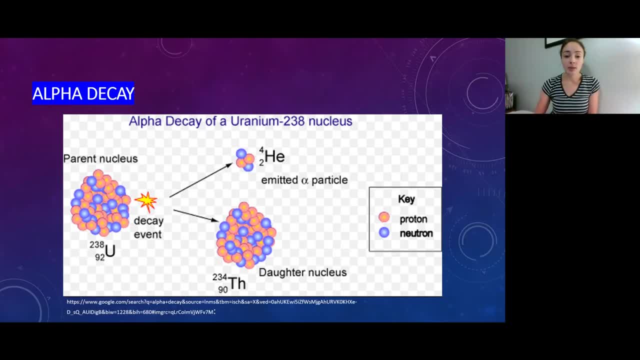 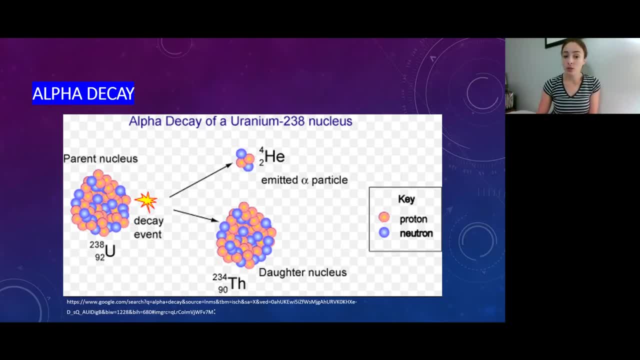 So it's decaying into thorium by losing a helium-232.. So it's decaying into thorium by losing a helium-232.. Or an alpha particle. or an alpha particle, like we talked about two protons, two neutrons. 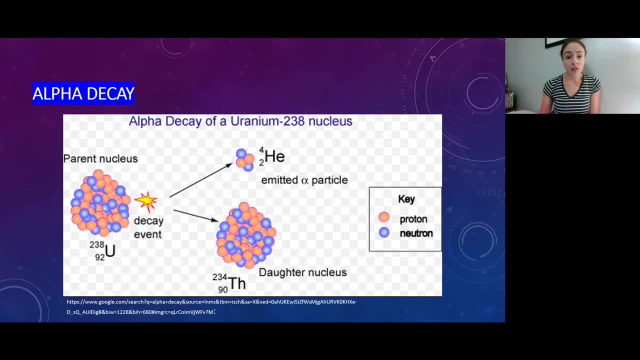 So therefore 238 becomes 234, because four particles from the nucleus aren't leaving, And then 92 becomes 90 because only two of those four particles are protons. In this slide you can see beta decay is depicted here in this figure as carbon-14. 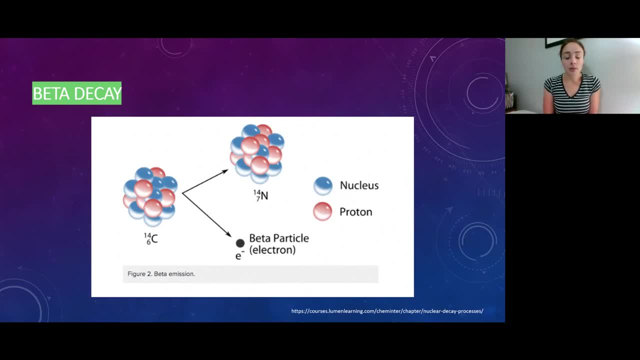 turns into nitrogen-14 by loss of a beta particle, turning one of the neutrons into a proton, which is why the proton number goes up, but the but the neutron plus proton number stays the same And in this slide you can see beta capture in this depiction. 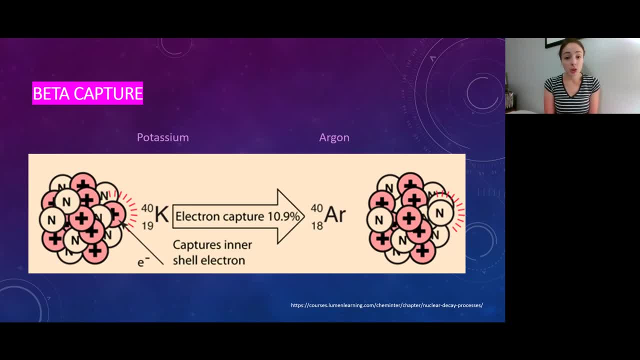 as potassium-40 captures one of its inner shell electrons, turning one of its protons into a neutron, causing the proton number to go down but the neutron plus proton number to stay the same, which causes the formation of argon-40.. 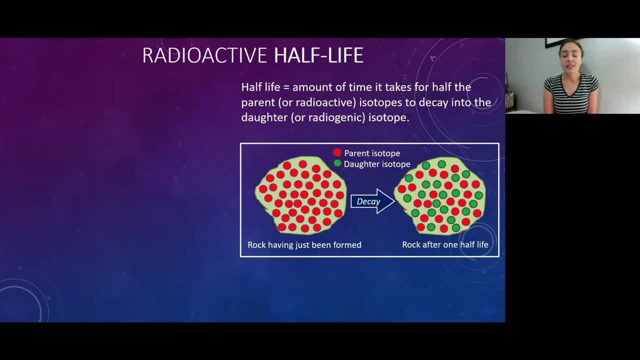 Okay, so half-lives. What are these half-lives? What does that mean, And how does that help us determine the age of the rocks? How does any of this help us determine the age of the rocks? Well, here we go. 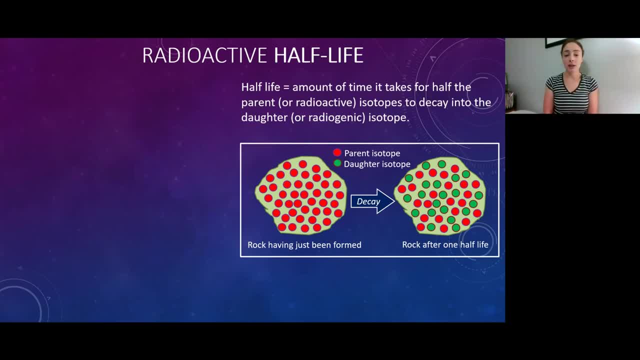 A half-life is the amount of time that it takes for half of the parent isotopes to decay into the daughter isotopes, And the parent isotopes are radioactive and the daughter isotopes are termed radiogenic. So you can see in this little diagram. 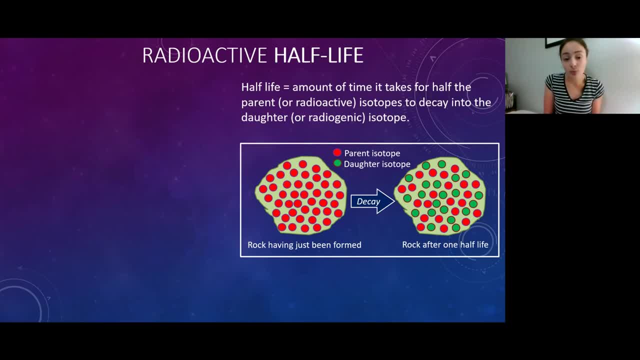 you have a rock that's just been formed, with 100% of its parent isotopes and 0% of daughter isotopes, whereas once it has decayed after one half-life, you will have 50% parent isotope and 50% daughter isotope. 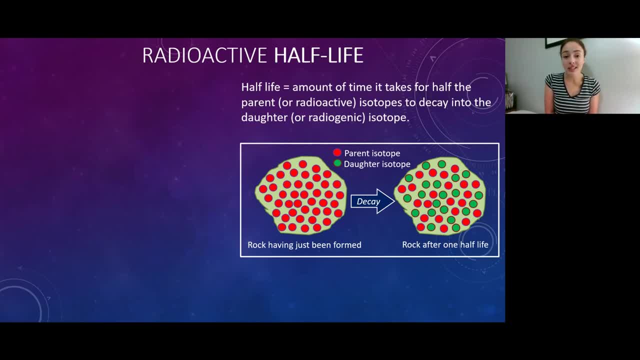 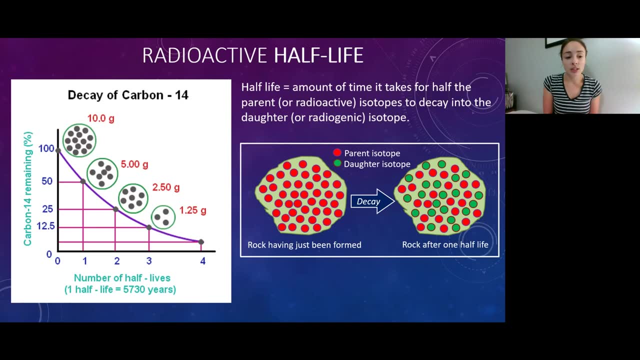 If you keep doing this, you will keep dividing the amount of parent isotopes in half, while the daughter isotopes will continue to accumulate. For example, we saw that the decay of carbon-14 happens by beta decay, but that doesn't matter here. 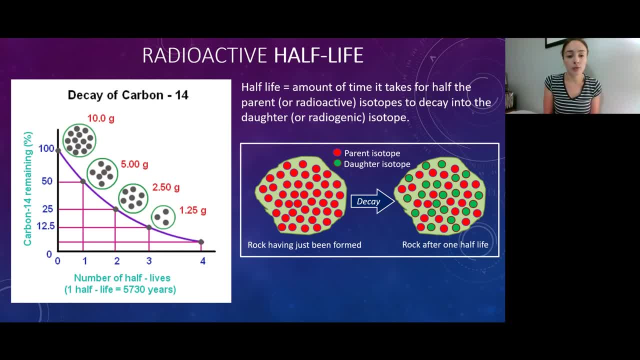 Basically, all you need to know is that the parent isotope is carbon-14, and that if you start with 100% of it and then one half-life goes by, you will get 50% of it, And if another half-life goes by, 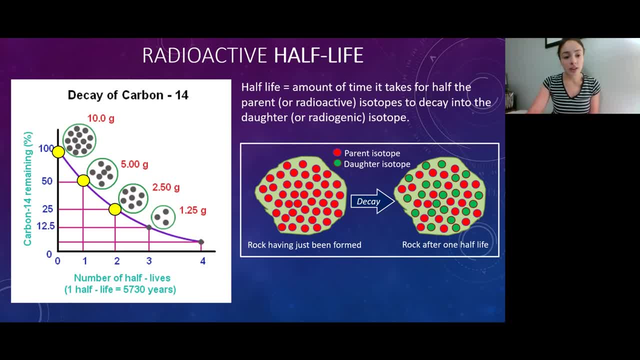 you will get 25% of it, And if another half-life goes by, you will get 12.5% of it, And if another one goes by, you will get 25% of it, And if another half-life goes by, you will get 12.5% of it. 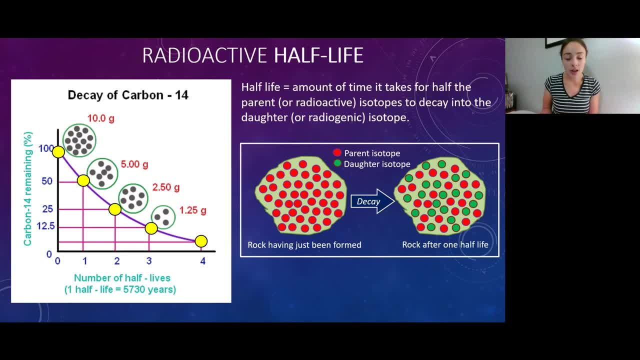 And if another half-life goes by, you will get 6.25% of it, And so on. This seems pretty simple, right? So how would you determine the age by this? Say, you come up to a fossil and you're like: 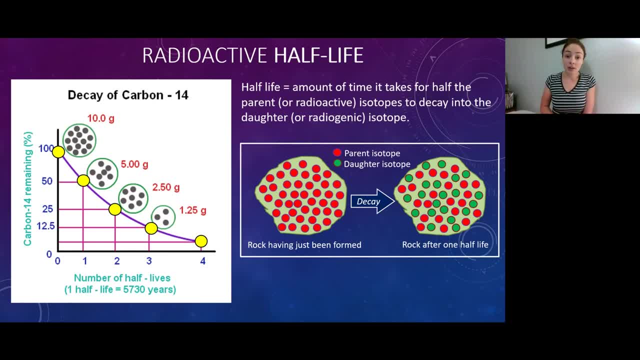 what is your age, man? And then you look at the amount of carbon-14 in it and you find that only 6.25% of the original carbon-14 is remaining. Then you know that four half-lives have gone by. 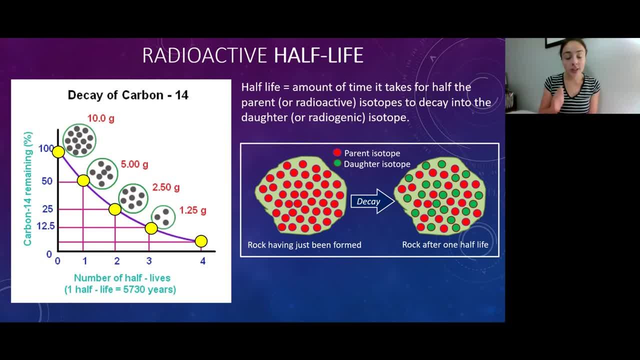 and you know the half-life of carbon is 5,730 years, because smart scientists have figured that out for us. You can multiply 4 by 5,730, and you will get the age of that fossil. But those of you with your brains screwed on today, 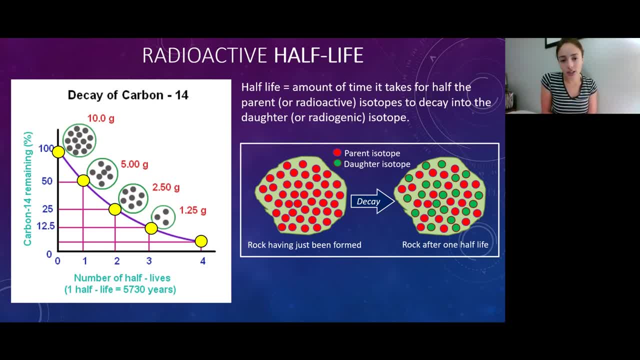 are probably thinking: how do you know that the amount of carbon-14 in there is only 6.25% of the original? How do you know the original amount? Well, you can deal with the daughter isotope. You take the ratio of parent to daughter isotope. 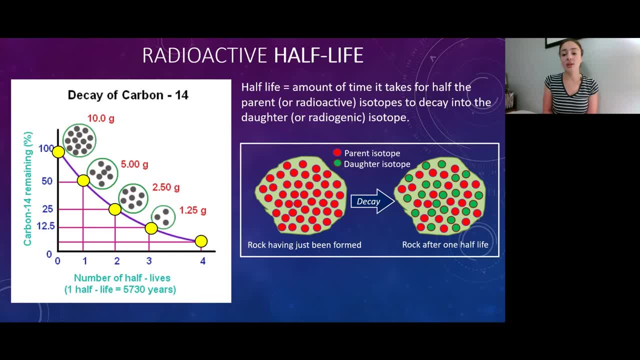 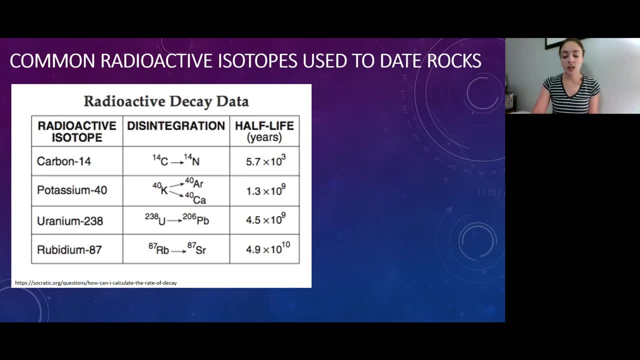 and you'll be able to tell not only how much parent is remaining, but also how much parent has decayed. Okay, so what can we use this on? Can we use this on all rocks? Not quite So. basically carbon-14,. you need to have organic material. 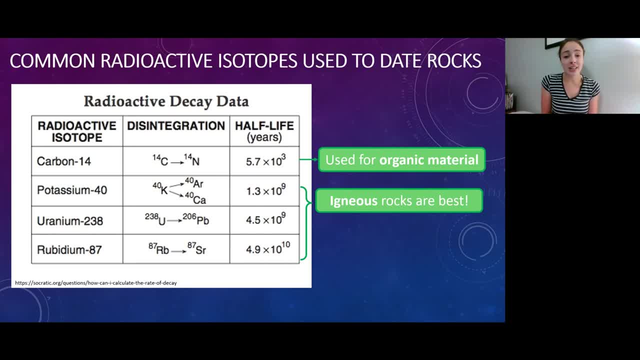 for pretty much all the other methods, you will need to have igneous rocks to be the most accurate, which is unfortunate, But you can also date metamorphic rocks if you're aiming for the last metamorphic event. Centimery rocks, however, are not as easy to date. 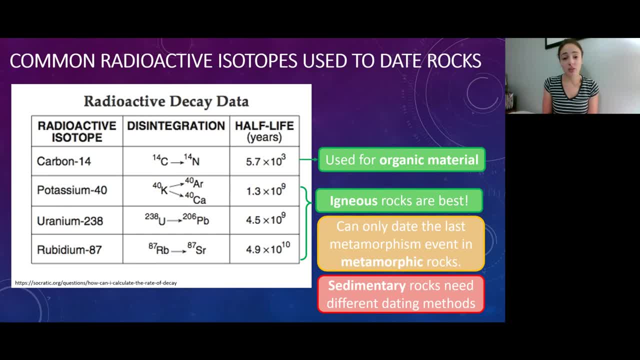 because their grains are just aggregates of previous grains from previous rocks, so you would get a different age from basically every single grain. There are some methods to determine the age of centimery rocks, such as something called optically stimulated luminescence. 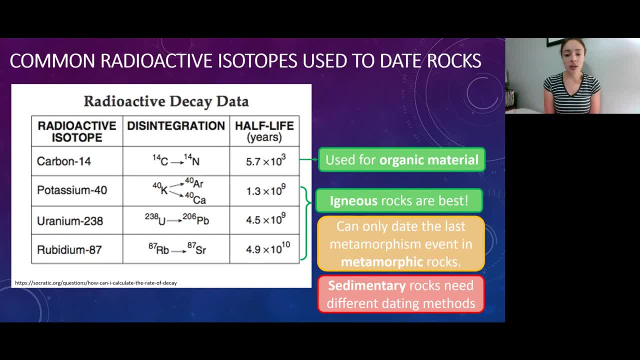 which I might describe in a future episode. Also, you can date seminary rock layers if you have enough fossils in them to relatively date them pretty accurately, or if you have layers of igneous material like volcanic ash layers, and sedimentary strata are often used to date formations of sedimentary rocks. 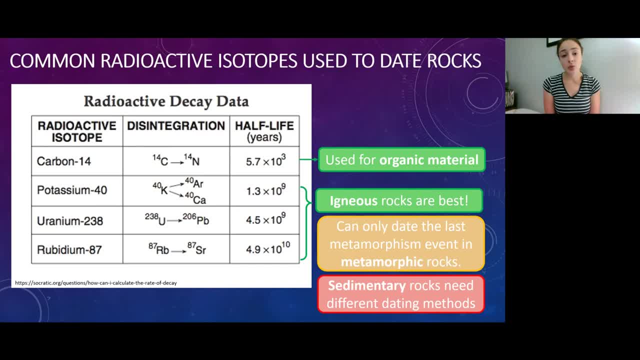 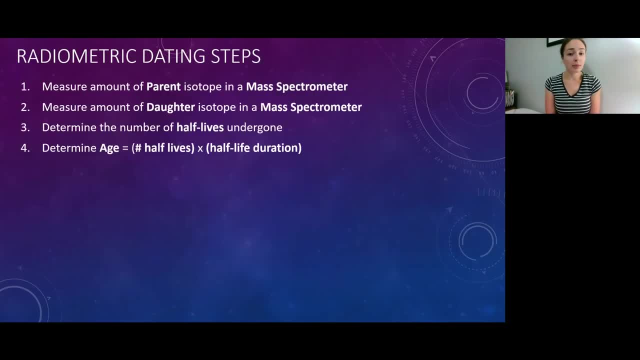 in a more precise way than maybe relative dating can get you. But all you need to understand here, basically, is the methods we described here worked best for igneous rocks. The way that you would apply radiometric dating is you would measure the amount of sedimentary rock layers. 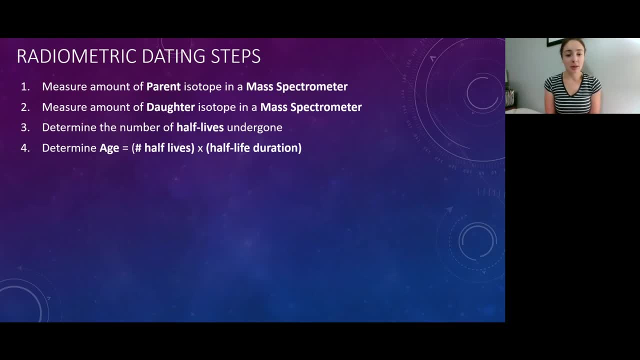 you would measure the amount of sedimentary rock layers, you would measure the amount of parent isotope in a mass spectrometer, you would measure the amount of daughter isotope in a mass spectrometer and then you would determine the number of half-lives. 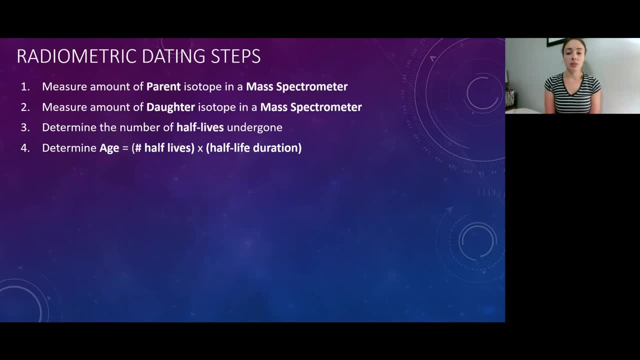 that have gone by this parent-daughter ratio, and then you would determine the age by multiplying the number of half-lives that have gone by, by the half-life duration that you know, because you can look it up Now. lastly, all I want to do here is do a couple examples with you. 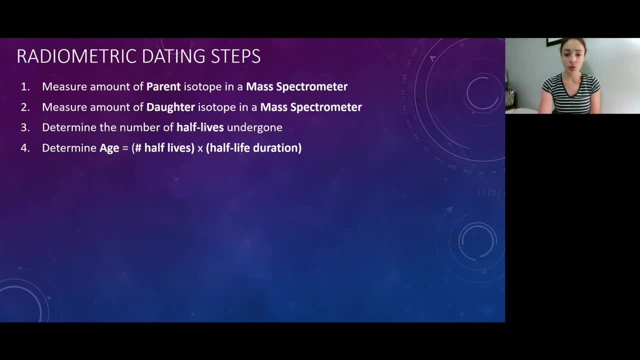 If you want to do some hands-on practice, you can pause before I tell you the answer and try it yourself First. a fossil bone is measured to contain 3.125 percent of its original C14 parent isotope. What is the age of the bone? 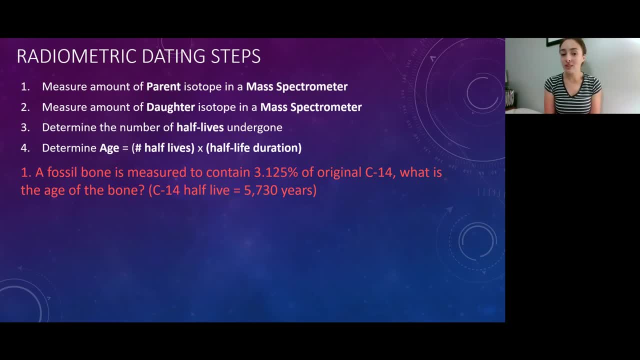 The C14 half-life is written down for your reference, so go ahead and pause the video and try it yourself. Now I'm going to tell you how I got the answer. Basically, the first step that I did was determine how many half-lives went by. 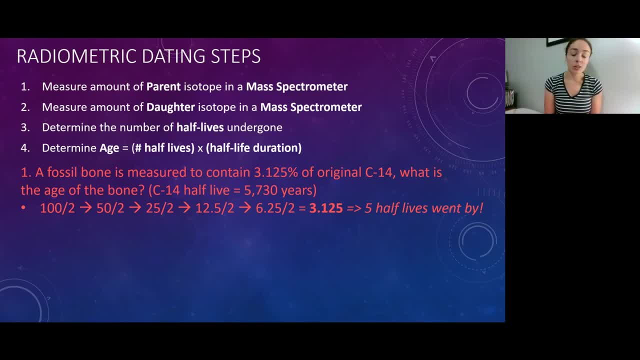 by starting with 100 percent of carbon-14, dividing by 2 until I got 3.125.. I got 3.125 after 5 times of dividing by 2, which means that 5 half-lives went by. And since I know how many half-lives went by. 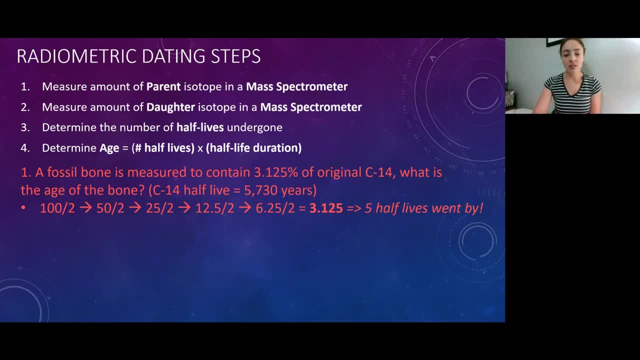 all I got to do is multiply 5 by 5,730.. This gets me 28,650 years of age. The second exercise asks: an isotope has a half-life of 6 hours. How much will be left after 24 hours? 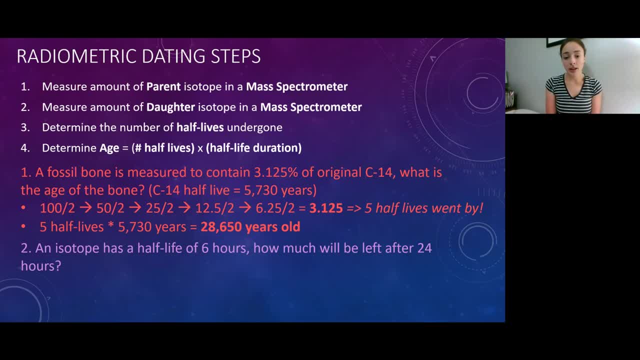 So to do this, first, I determined how many half-lives would go by after 24 hours. Basically, how many times can you put 6 hours into 24 hours? And that is 4.. So I'm at a table and I'm going to put 4 half-lives into 24 hours. So I'm at a table and I'm going to put 4 half-lives into 24 hours. I'm at a table and I'm going to put 4 half-lives into 24 hours, 4 half-lives with 2 rows. 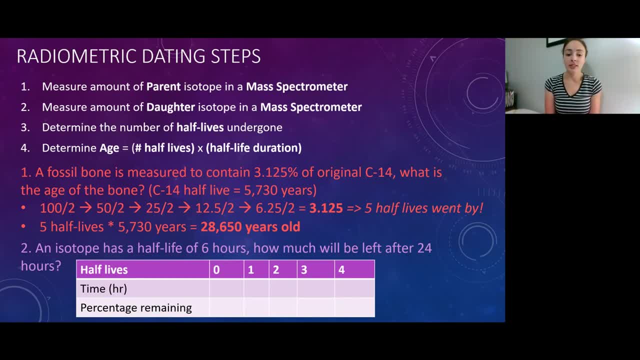 First row is time, second row is percentage remaining, and this is the most clear and easy way to do this problem. So at time, 0,, 0 time has gone by and 100 percent of the parent isotope is remaining After the first half-life. 6 hours have gone by. 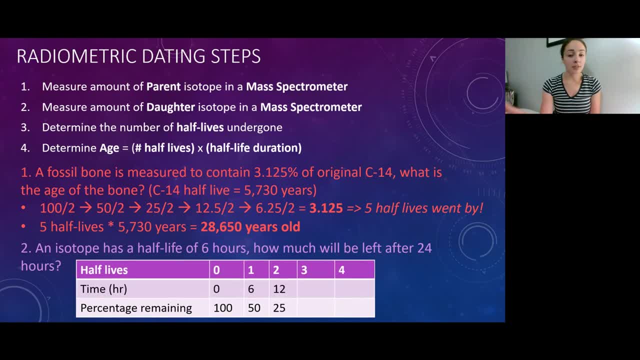 and 50 percent of the parent isotope is remaining After half-life 2,. 12 hours have gone by and 25 percent is remaining After the third half-life: 18 hours have gone by and 12.5 percent is remaining. 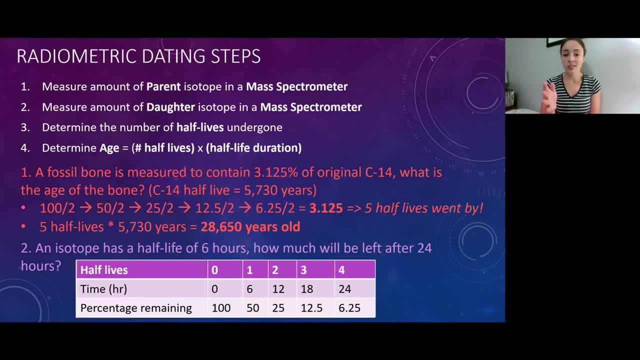 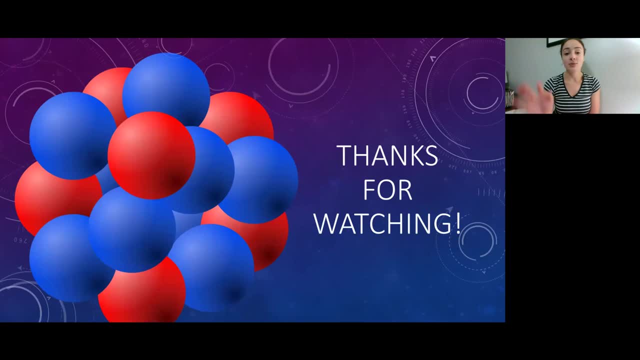 remaining, and after the fourth half life, you are at your end of your 24 hours and 6.25 percent of your parent isotope is remain. so i hope this practice helped and i hope this video helped, and i hope you guys enjoyed learning about absolute dating as much as i enjoy anything. 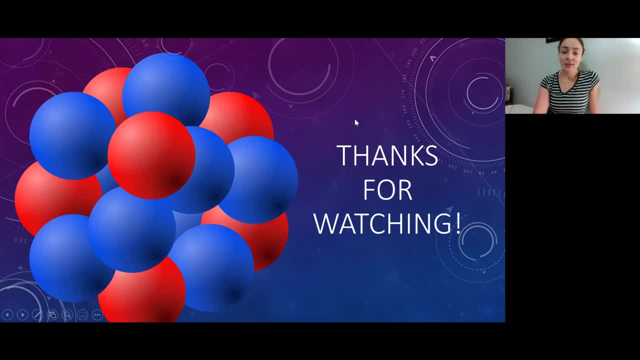 that has to do with isotopes. thank you so much for watching and i will see you all next time.